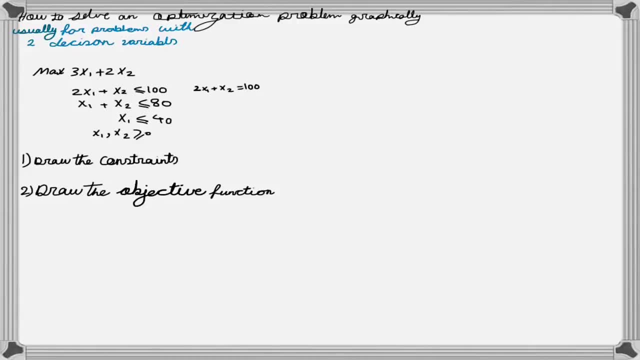 Now, to draw a line in a two-dimensional space, we need two points. We usually find these two points by one, setting x1 equal to 0 and one setting x2 equal to 0. For this line, if I put x1 equal to 0,, 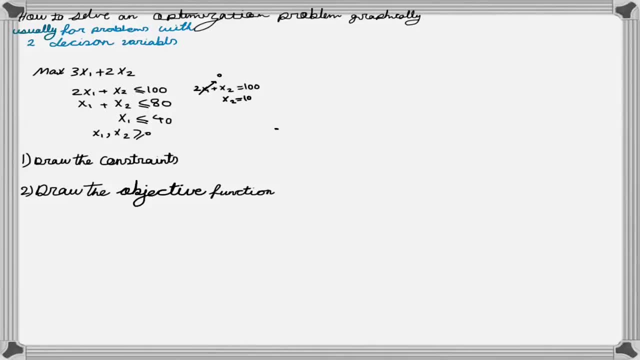 then x2 will be equal to 100, and if I put x2 equal to 0, then x1 will be equal to 50.. Now, having these two points, I'm able to draw a line represented by these two points. 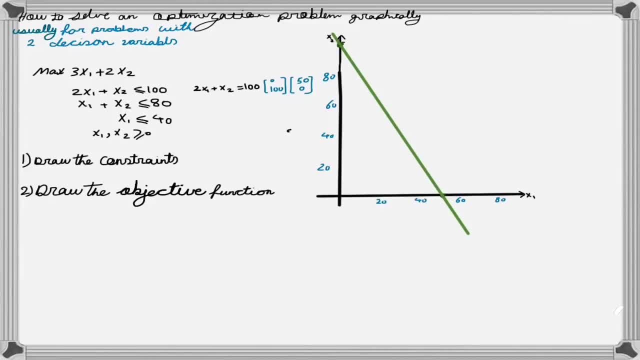 Okay, if I find the two points and then connect the two points that are given here, I'm able to draw this line. Now, to check what side of this line I'm looking at in this inequality, one way is to pick an arbitrary point which is not on the line. 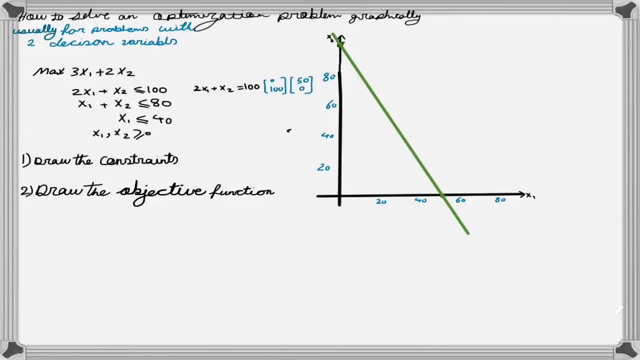 and see if it satisfies the inequality or not. If it does, we are looking at the side that includes the point. Otherwise, we are looking at the opposite side. By standard, we usually select the points 0 and 0 if it's not on the line. 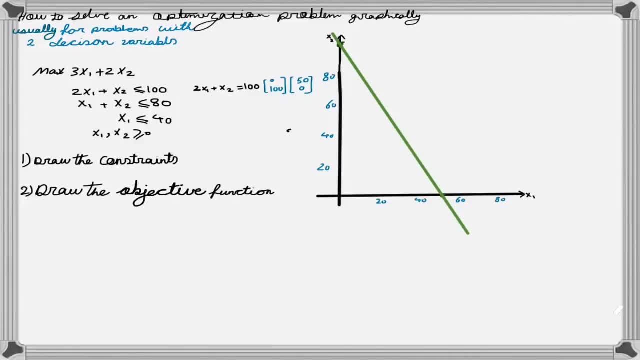 And in this example, if I select point 0 and 0, which is the center of the coordinate here. now, if I put this point in the first constraint and replace x1 and x2 by 0, you see that 0 is less than 100,. 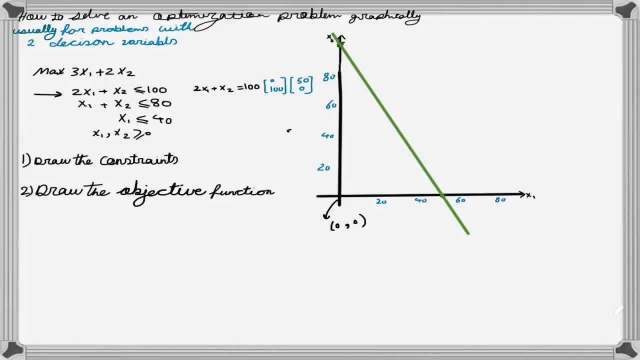 so the constraint is satisfied. so we are looking at the side that includes the points 0 and 0.. We can show this conclusion with an arrow on the line Now, if I draw the second line of this problem again by setting x1 and x2 equal to 0,. 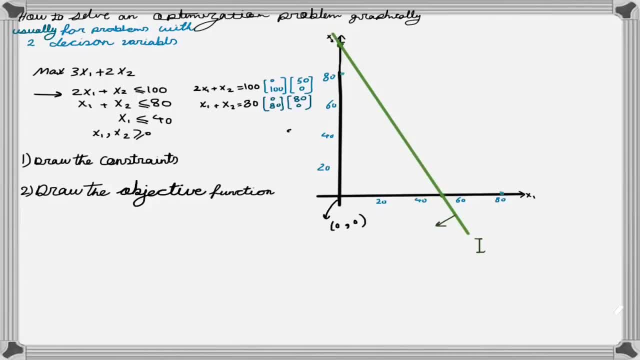 I'm able to find two points where, if I connect these two points, I can get the second constrained line. Now to decide what side of this line we are looking at, and this inequality, again, we can replace the points 0 and 0. 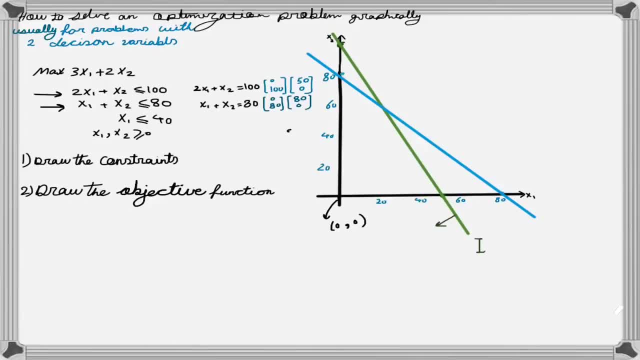 in the second constraint and check whether the condition is satisfied or not By replacing 0 and 0, the condition is true, so we are looking at the side that includes 0 and 0. Remember to name your constraint as you move forward. 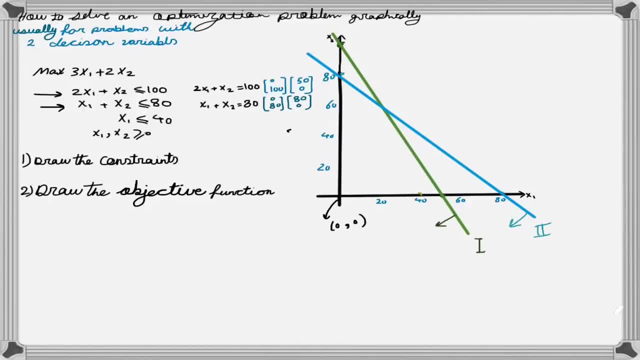 because later on we might be interested in finding the intersection of lines and it makes your life easier to know what lines you are looking at or what is the line equation that you need to pick to find the intersection point. Now, the last constraint is x1, less than or equal to 40. 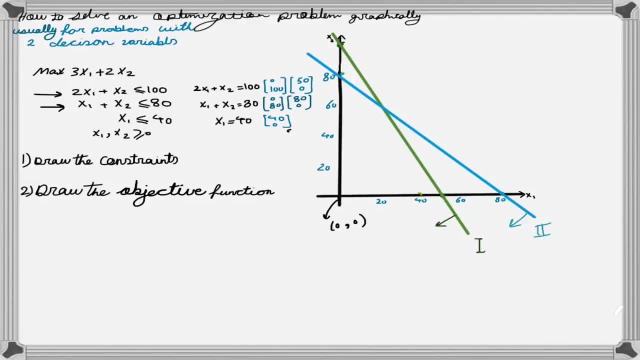 and for this line it's enough to find one point, which is 40 and 0. And we are looking at the side that includes the points 0 and 0, because if we put x1 equal to 0,, 0 is less than 40. 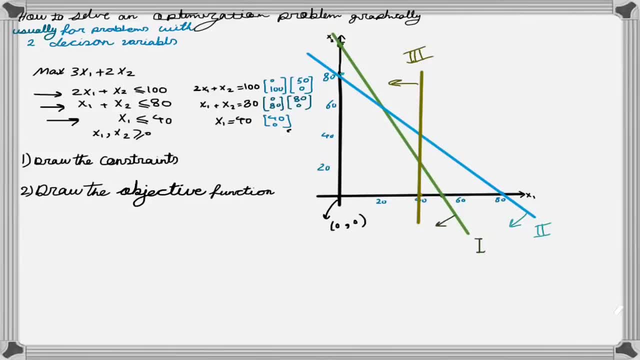 and the condition is satisfied in this constraint. Now we are done with drawing our constraints, we can form the feasible region, which is, in fact, the intersection of all the areas found by constraints. The intersection of all these feasible areas will be the area that is shown by yellow. 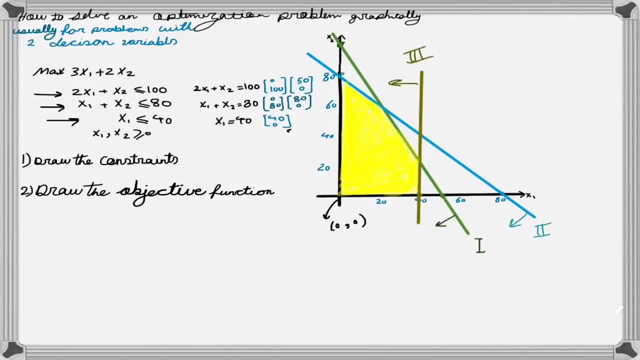 in this example. Now that we are done with finding the feasible area, we are interested to find the x1 and x2 in this area. that maximizes the value of objective function, which is 3x1 plus 2x2, and this is the meaning of optimization. 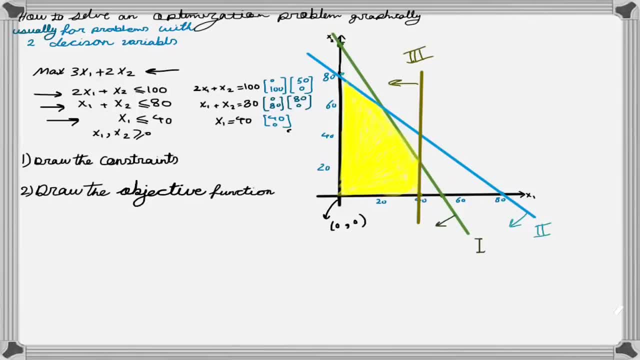 We have a feasible area. we have a lot of alternative for x1 and x2. Any points in this region is a feasible solution to our constraints. Now we want to find the combination of x1 and x2 that maximizes this function here. 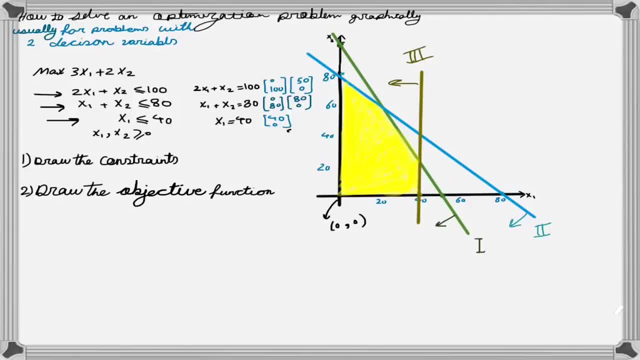 To be able to find the point that maximizes this function, we start by putting the objective function equal to some arbitrary number. This arbitrary number is 60. You can put this function equal to any number that you would like, But in this example I selected 60.. 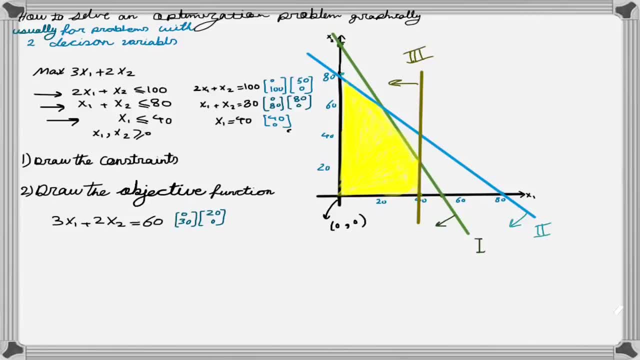 The next step is to draw this line Again. by setting x1 and x2 equal to 0, we can find two points and by connecting these two points we are able to draw the objective function line. Please note that the value of objective function. 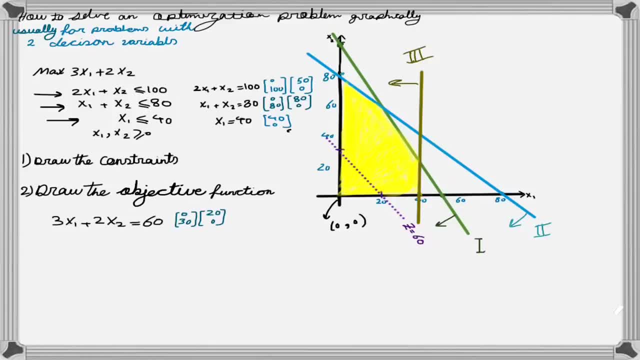 for all the x1 and x2 on this line will be equal to 60. So any single points on this line have the same objective function, which is z equal to 60.. Now that we draw the objective function line, we need to repeat this step. 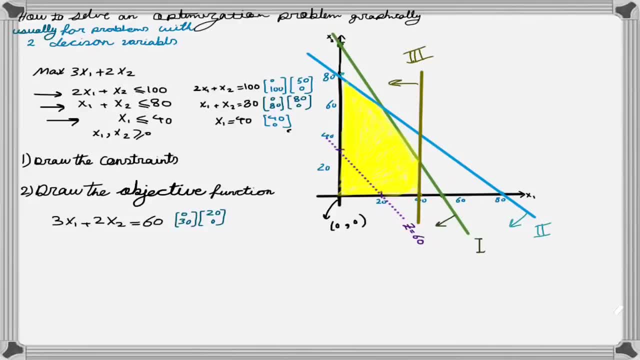 but this time we set objective function equal to a different number. Defining the new number is dependent to the objective function direction. By direction I mean whether we are looking at a maximization or a minimization objective function. If you are looking at the maximization problem, 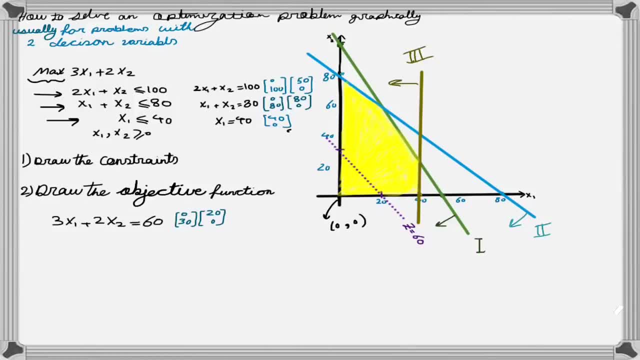 the second point or the second value that you select for your objective function should be greater than the initial points that you have selected. Since in the first try I selected 60 and I am looking at a maximization problem, my second value should be greater than 60.. 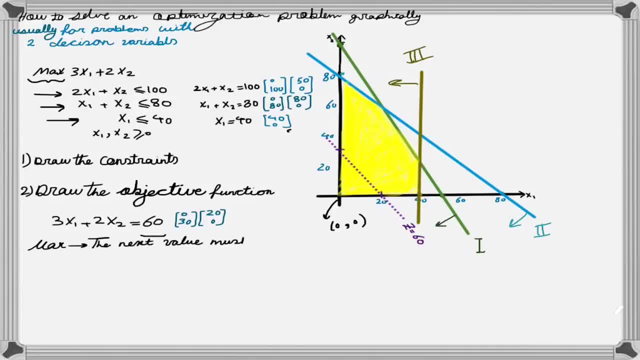 So for a maximization problem, the next value must be greater than the initial value of 60 that I selected. But if I was looking at a minimization problem, the second value or the next value that I select for my objective function should be lower than 60.. 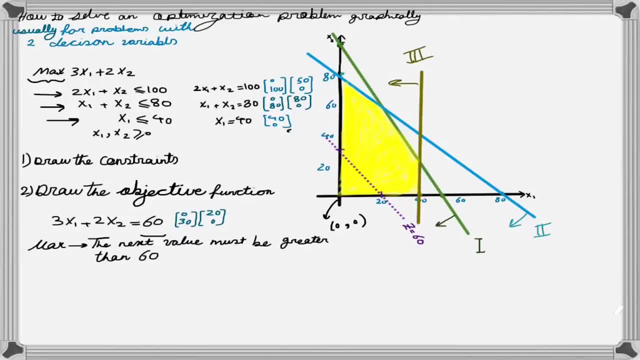 Something like 40 should be my choice for a minimization problem. So remember, for a maximization problem, the next value always greater than the initial value, and for a minimization problem, the next value always less than the initial value. Now the next value that I selected. 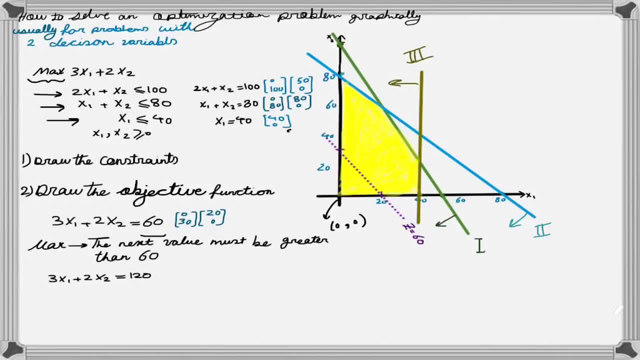 in this example is 120.. Now I need to draw this line as well. So I select two points by setting x1 and x2 equal to 0, and if I connect these two points, I get the line for z equal to 120.. 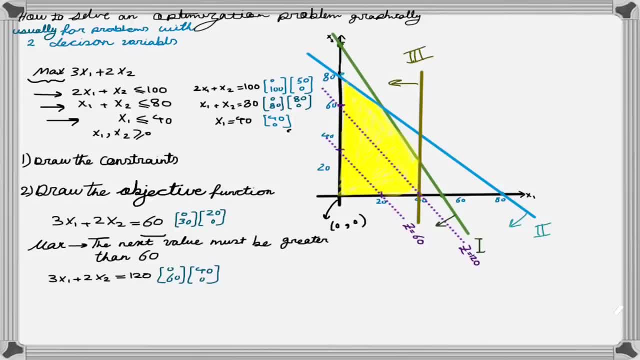 Again, note that all the points on this line have the same objective function of 120.. The two lines, z, equal to 60, and z, equal to 120, are parallel lines And as we increase the objective function we are moving toward the right-hand side. 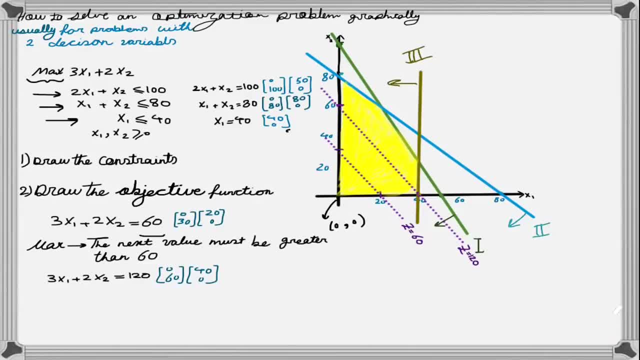 of this plane. As you see, if we move the objective function line to the right-hand side, parallel to the initial objective function line, its value will increase. This shows the direction of improvement for the objective function. According to a theorem in a convex set. 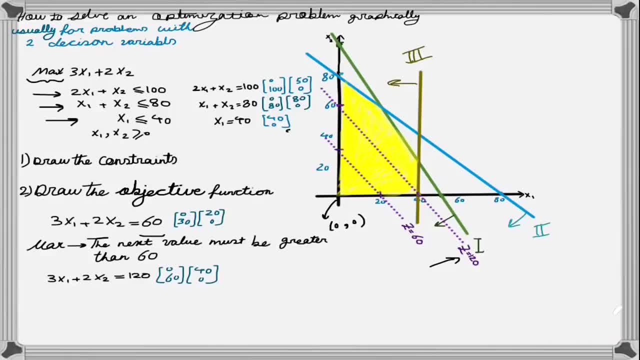 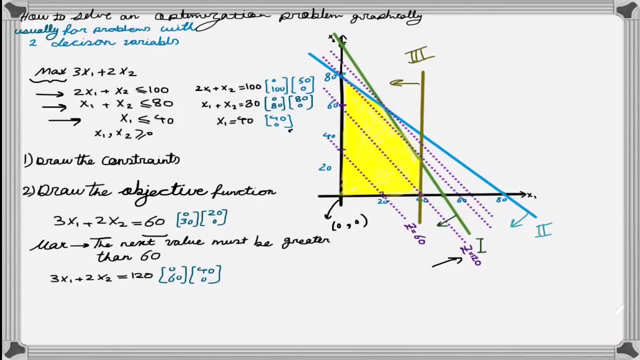 the optimal solution happens at the last corner of the feasible area that objective function line hits as it's moving toward its improvement. Improvement in a minimization problem means a reduction in the objective function and for a maximization it means an increase in the objective function. 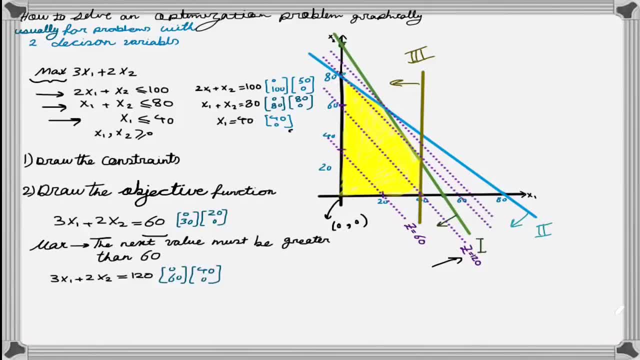 Since we are looking at a maximization problem. improving the objective function is synonym to an increase to its value. As you see in this example, the last corner point that the objective function hits as it's moving, the feasible area is this point. The optimal solution is at the intersection. 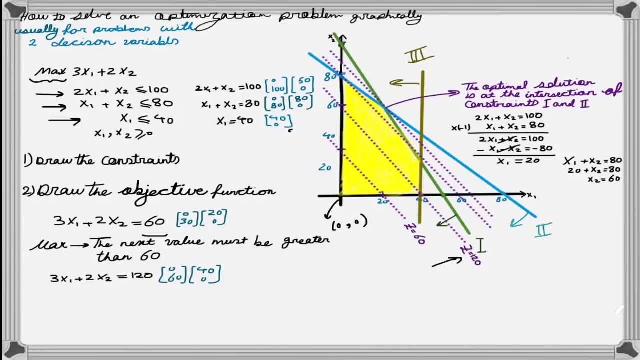 of constraints 1 and 2.. Now we have to find the intersection of these two points. By solving the equations for the intersection, we'll find x1 equal to 20 and x2 equal to 60 is the optimal point for this problem. 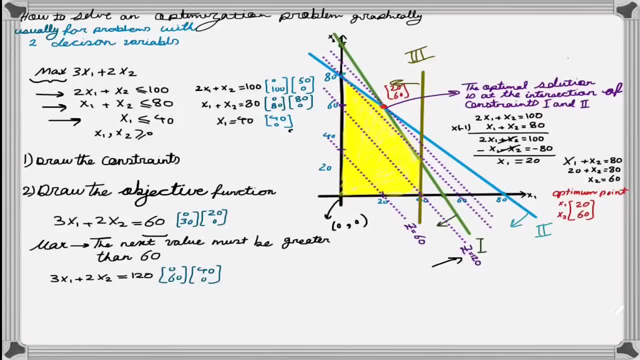 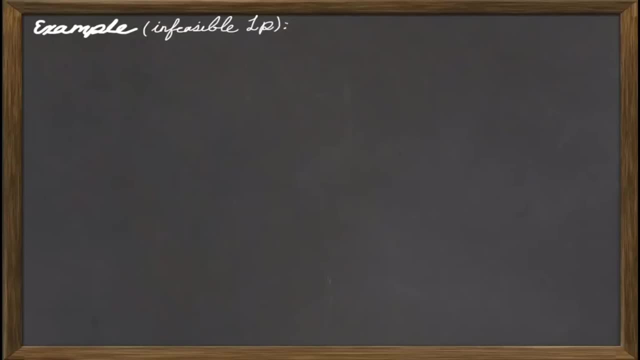 Now we have to find the value of objective function for the optimal solution. By replacing x1 and x2 in the objective function, we get the value of z equal to 180, which shows the optimal solution to this problem. Sometimes there is no feasible solution. 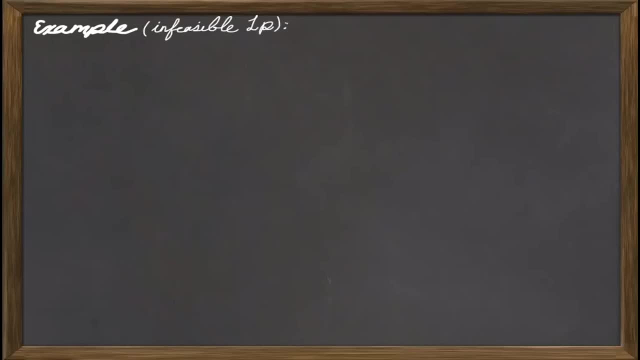 for a linear programming problem. In this part we take a look at an example of an infeasible LP. Suppose we have a maximization problem, as shown on this screen. Now let's draw the constraint and form the feasible area for this problem. 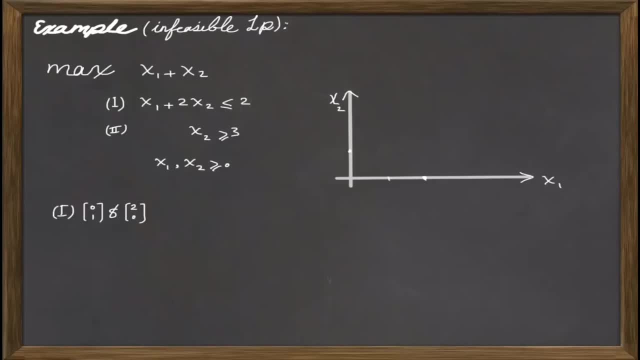 For the first constraints, if we set x1 and x2 equal to 0, we are able to find two different points where, if we connect the two points, we find the first constraint of the problem To decide what side of this line we are looking at. 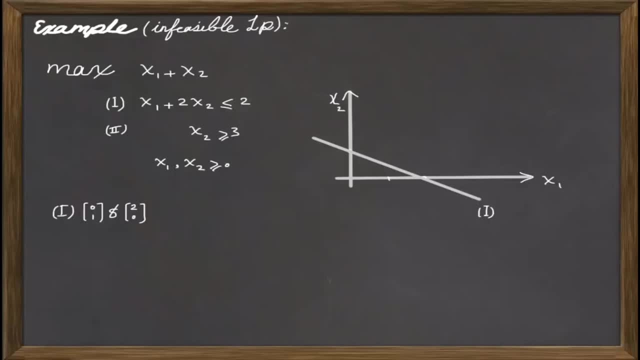 we need to replace the point 0 and 0 in the first constraint, Since the first constraint is satisfied with this point. we are looking at the side that contains the value of 0 and 0, which is this side. Now, if I look at the second constraint,